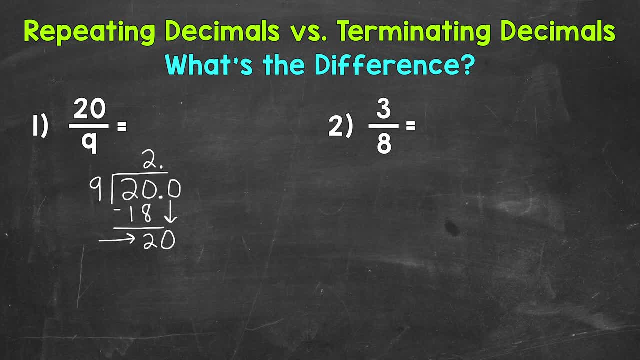 continue on forever and you'll see a pattern. So let's see what happens here: 20 divided by 9.. Well, that's 2.. 2 times 9 is 18.. Subtract, We get 2.. So we need to continue on. We'll use another zero. Bring that down. 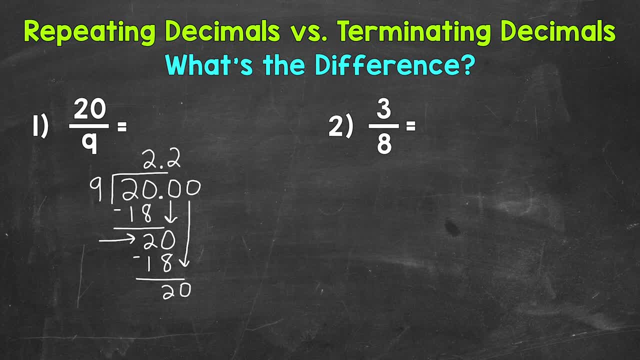 So we have 20 divided by 9 again, which is 2.. Let me extend this bar here 2 times 9 is 18. And you'll probably notice a pattern. So 20 minus 18 is 2. We'll use another zero And this pattern is going. 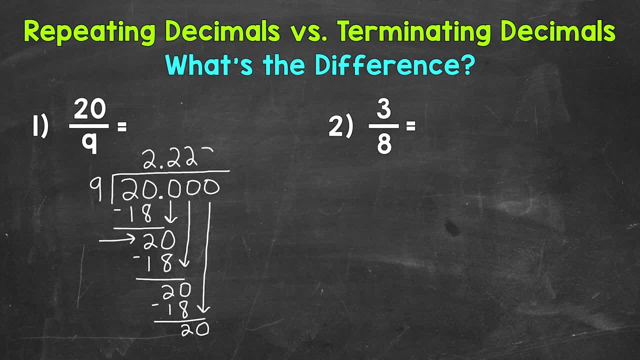 to continue on forever. So how many 9s out of 20? 2. 2 times 9 is 18.. I ran out of room there, but 20 minus 18 is 2.. We would bring down another zero. 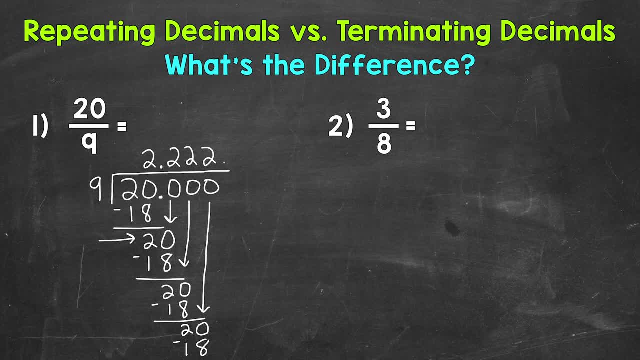 And again, that pattern is going to continue on forever. So this is a repeating decimal. We will have 2s that go on forever. So we can write our answer like this: 2, decimal 2, and then put a bar above the decimal portion that repeats. So we have a 2 that repeats. So put the bar above the 2. 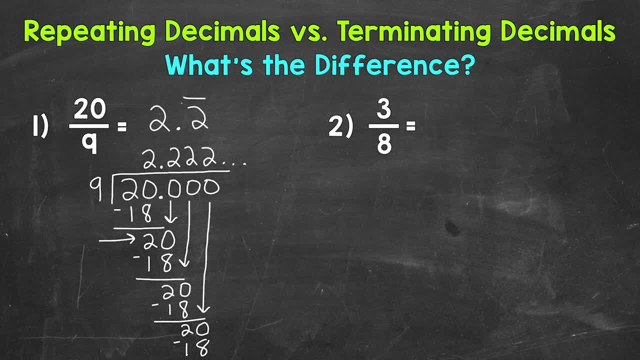 and that shows that we have a repeating 2.. This is called bar notation. So our final answer: 2 and 2 repeating. Let's move on to number 2, where we have 3 eighths or 3 divided by 8.. Let's set: 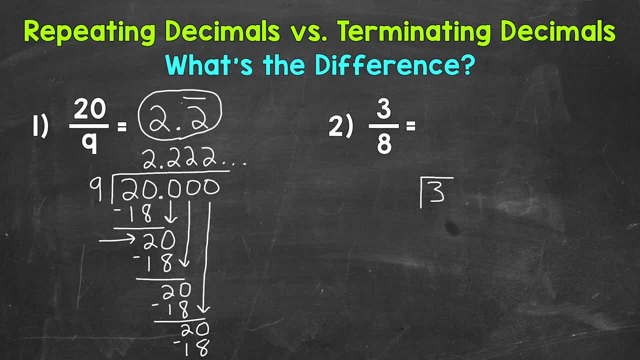 this up. So 3 divided by 8. How many whole groups of 8 out of 3?? Well, we can't do that, So we can put a zero here. We want this in decimal form, So let's place it after the whole number and bring. 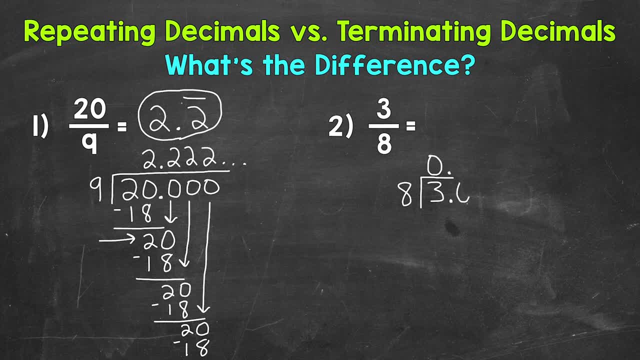 it straight up into our answer: We will use a placeholder zero to continue through our division process. So 30 divided by 8. How many whole groups of 8 out of 30?? Well, 3. That gets us to 24.. 3 times 8., 24. Subtract, We get 6.. So we did not get a clean cut zero yet. So